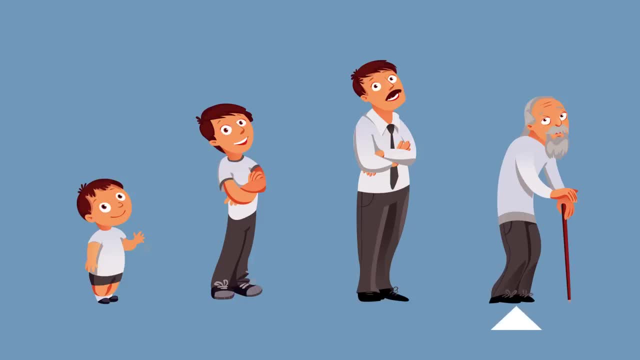 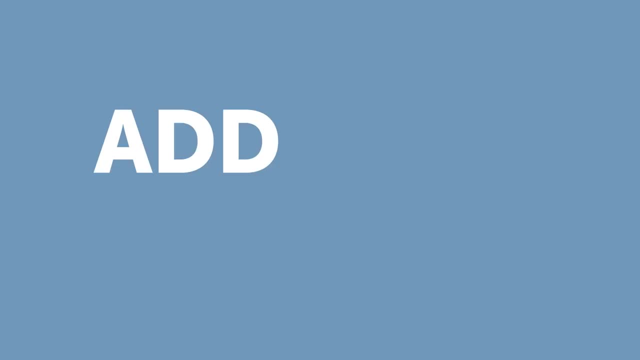 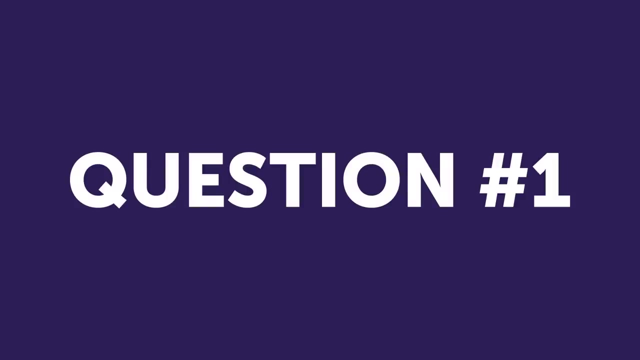 you're a carefree child, an old, wise sage or just exactly as mentally old as you are. Just answer our questions, write down your points for every answer, add them all up and get your results. But enough talking, Let's begin Question number one. Look at this picture. 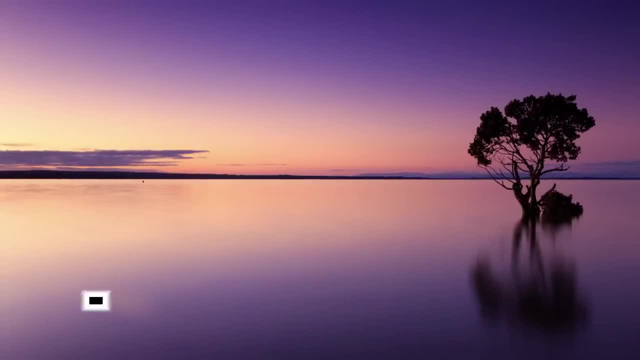 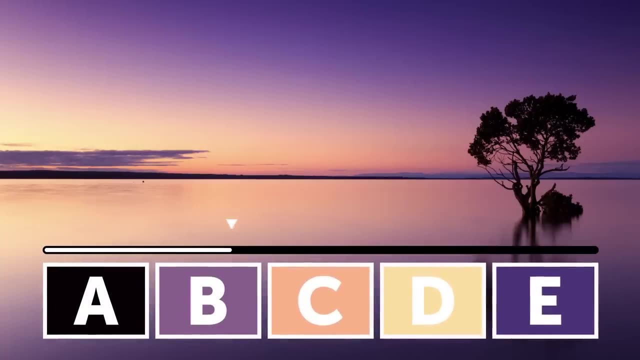 In your opinion, which color is dominant here? You have five options here: A, B, C, D or E. If you chose A, it's four points. The answer B equals five points If you saw C as the dominant. 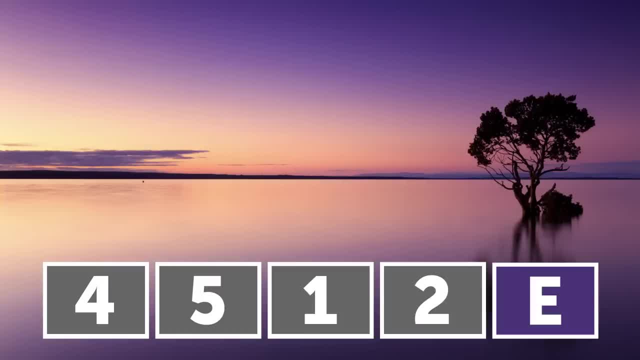 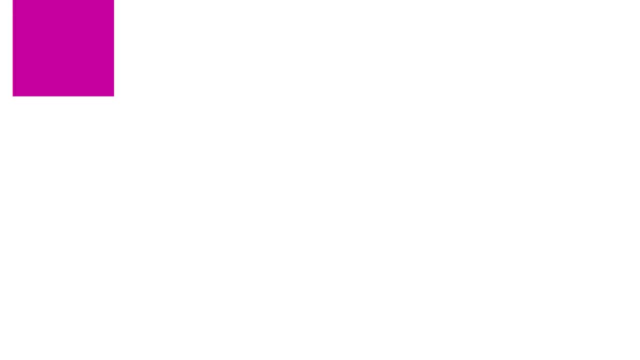 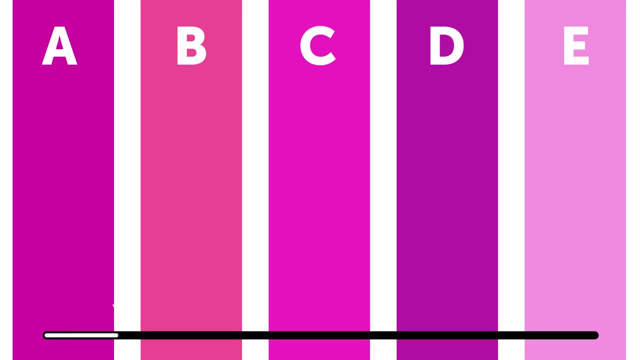 color, it's one point. Color D gives you two points and E means three points. Question two: Here we have five beautiful shades of pink for you. Which one do you like the most? If you preferred shade A, add three points. Shade B leaves you with two points. If your. 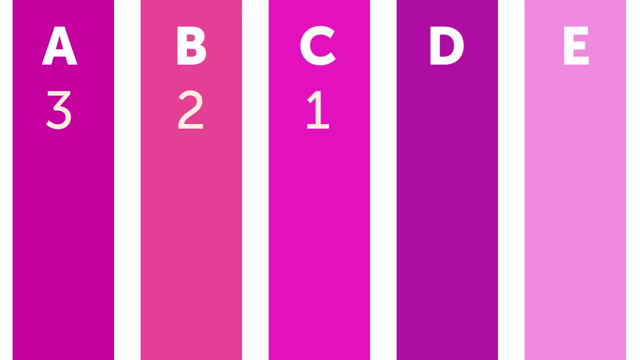 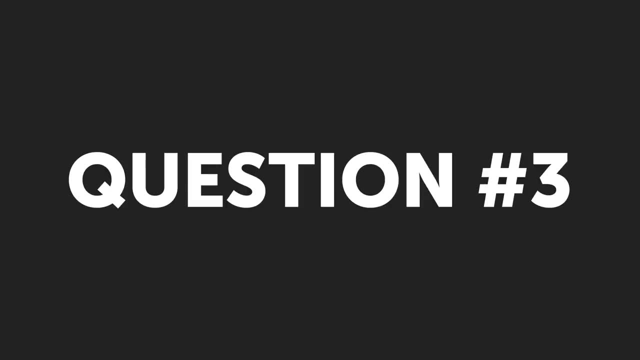 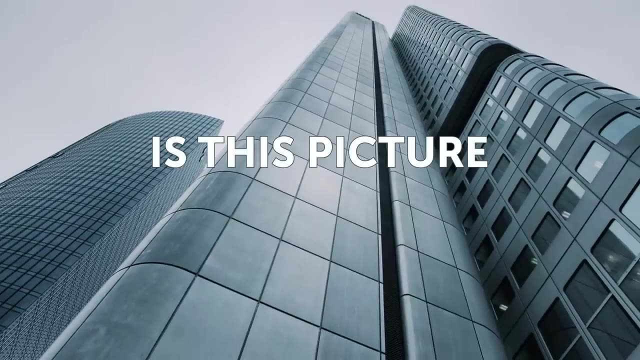 favorite is C, you'll get one point. Pink shade D equals five points, while for E you have to write down four points. Question three: Look at this beautiful photo. We have just one question for you: Is this picture black and white? 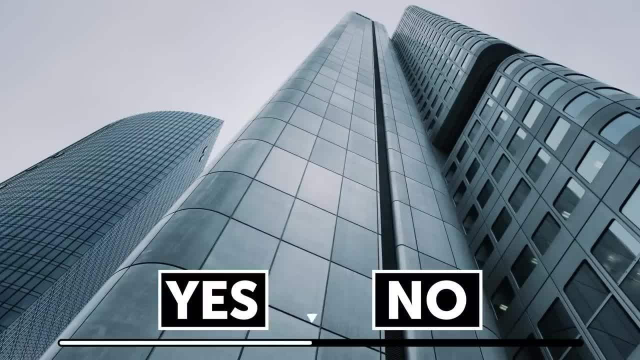 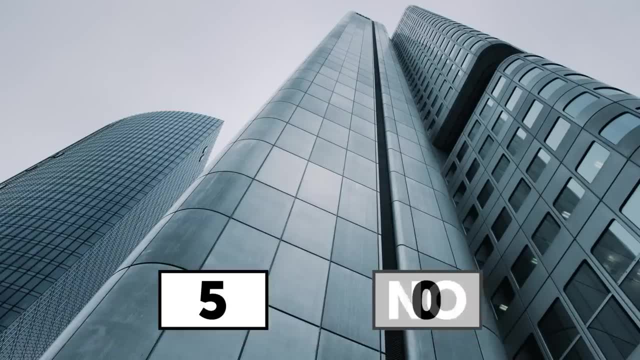 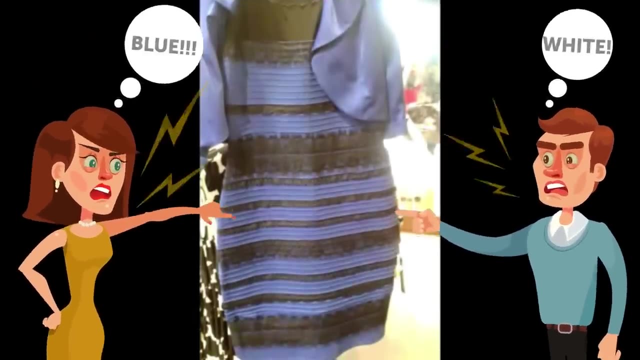 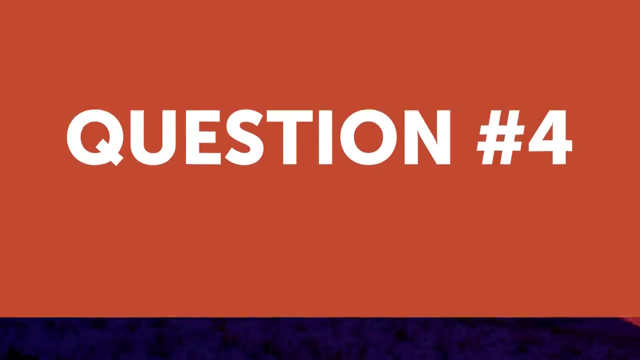 If you think that it is, add five points. If not, don't add anything. Man, I hope it won't start a huge debate, like with this blue and white dress. Remember that. Anyway, another question is waiting for you, Question four. I hope you like sunsets, just like I do, So here's four pictures of a couple of the 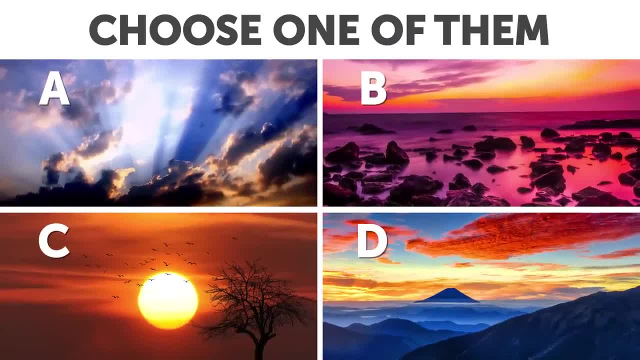 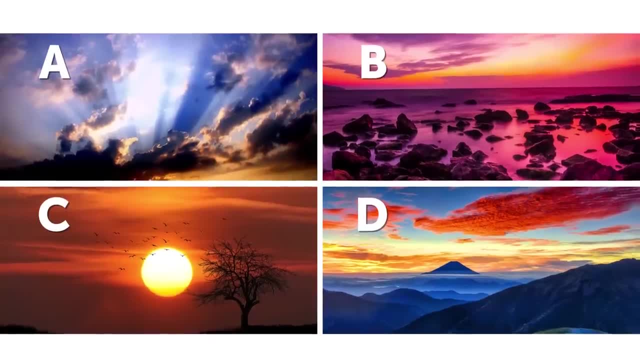 most beautiful sunsets I've seen in my life. Here's a picture of a couple of the most beautiful sunsets I've seen in my life. sets ever. Choose one of them If the first sunset is. so you add 3 points If you got. 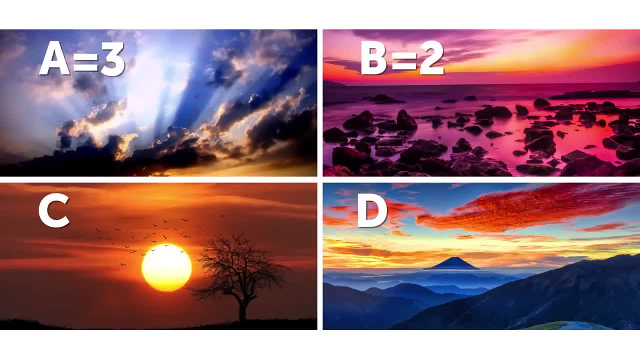 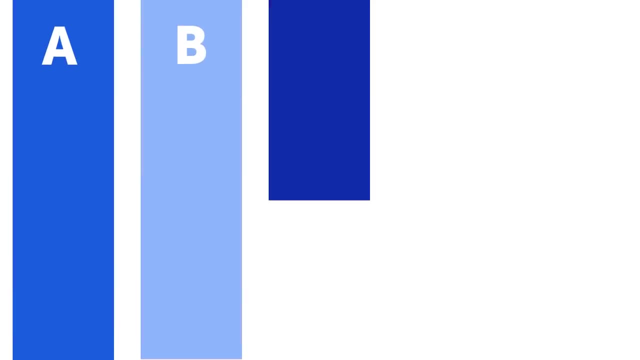 too distracted by the second one, you get 2 points. The beautiful third option gives you 4 points And finally, sunset number 4 leaves you with 1 point, Question 5.. Now that we're done with the shades of pink, let's do the same thing. 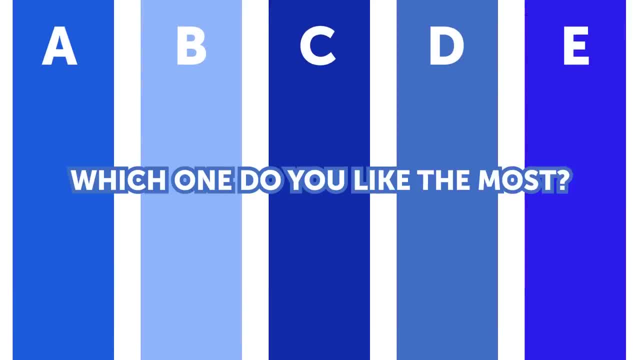 with the shades of blue. Which one do you like the most? Shade A gives you 2 points. Dreamy B equals 4 points. For C, write down 3 points. D stands for 5 points and E means… yep, 1 point. 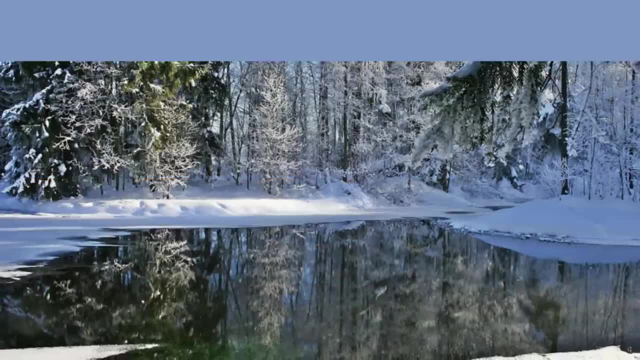 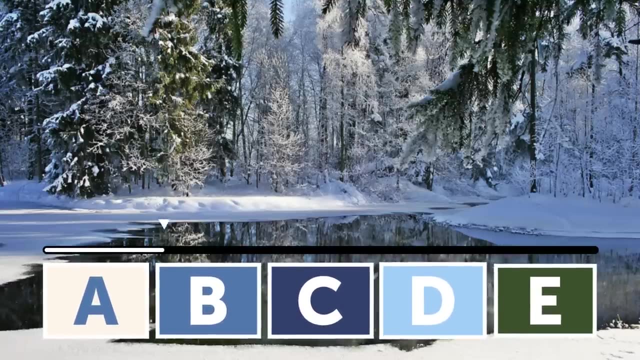 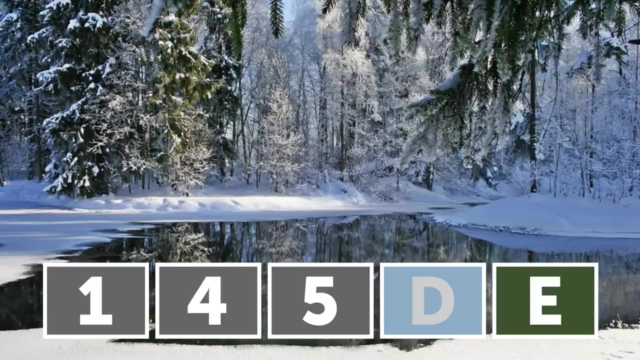 Question 6.. Here's the beautiful winter view. Which color in this picture did you see first? White gives you 1 point. Option B is 4 points. If you chose C, add 5 points. D and E mean 3 and 2 points respectively. 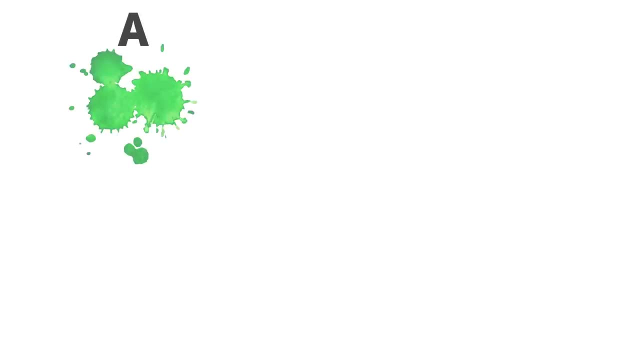 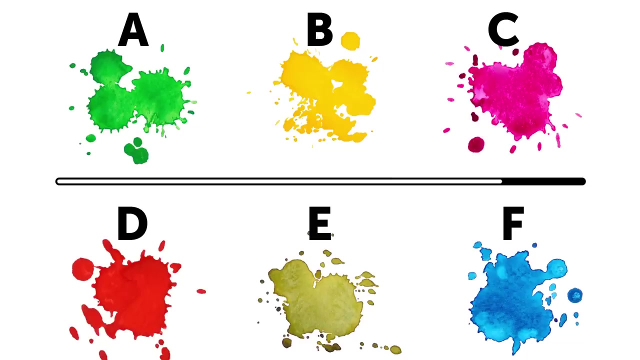 Question 7.. Let's go, Let's make it a little easier. Choose a watercolor. If green A is your favorite, write down 2 points. Yellow B gives you 4 points. Pinky C stands for 5 points. Red D leaves you with 1 point. Original E option equals 6 points. 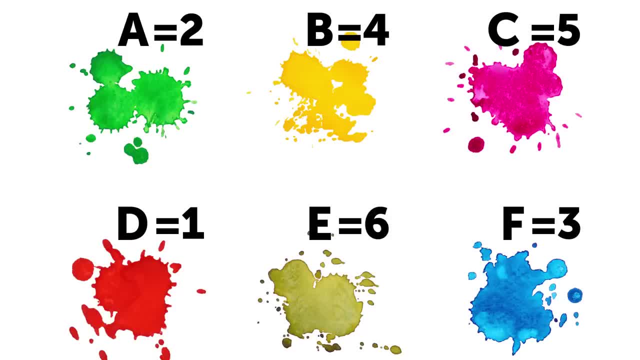 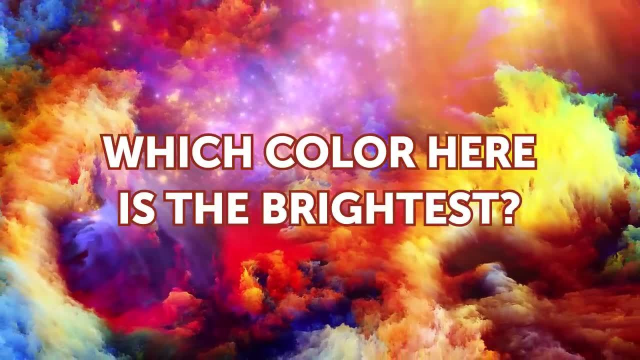 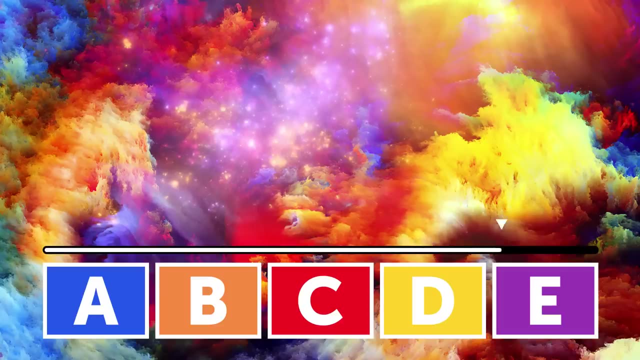 and bluish F adds 3 points to your current number, Question 8.. Look at this picture. Which color here is the brightest? If you chose Option A, 4 points for you. B gives you 2 points. Red C is for 1 point. 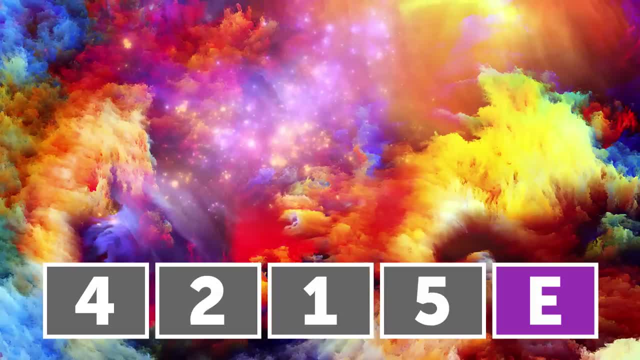 while D gives you 5 whole points. Finally, E equals 3 points, And that was the last question Time to answer the next question, Question 8.. Look at this picture. Which color here is the brightest? Red C is for 1 point. 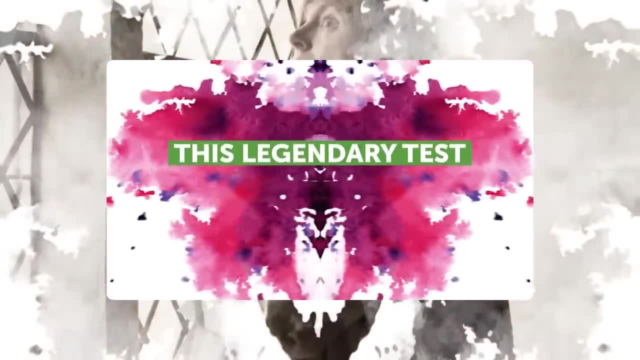 while D gives you 5 whole points. Finally, E equals 3 points, And that was the last question, Question 9.. Let's go with a purple one. Let's add up all the points. By the way, if you want to find out even more about yourself, check out another cool test. 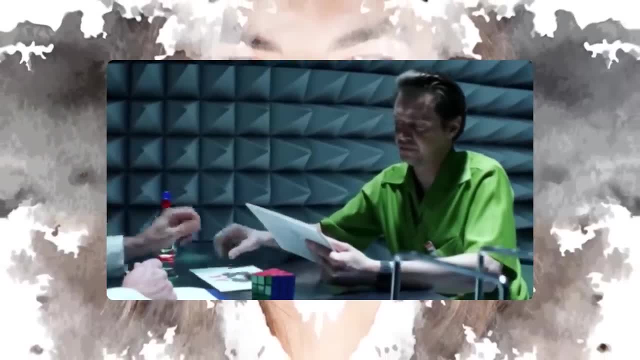 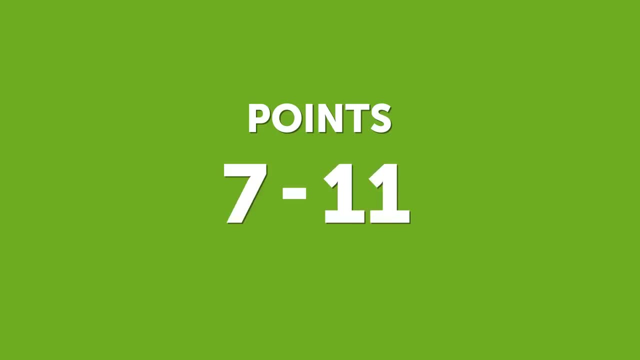 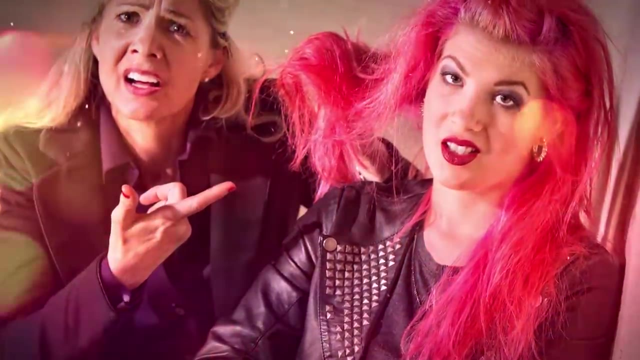 right here. It will reveal the deepest truth about your character. But back to our test. Results are finally here. If you got 7 to 12 points, mentally you're just under 20 years old. It doesn't matter what your passport says – you're a carefree teenager at heart. 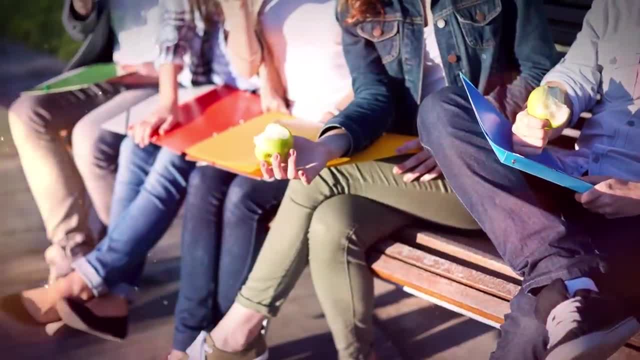 If you're way older than 20, congratulations. You've managed to carry this constant burden. If you've got a girl over 30 years old, you've got a girl under 20 years old. You've got a girl over 30 years old. You've got a girl over 30 years old. You've got a girl over 30. 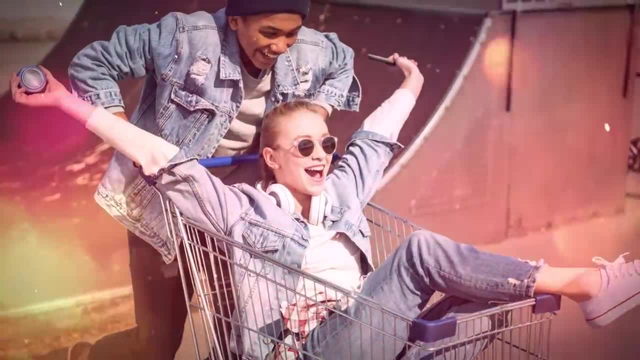 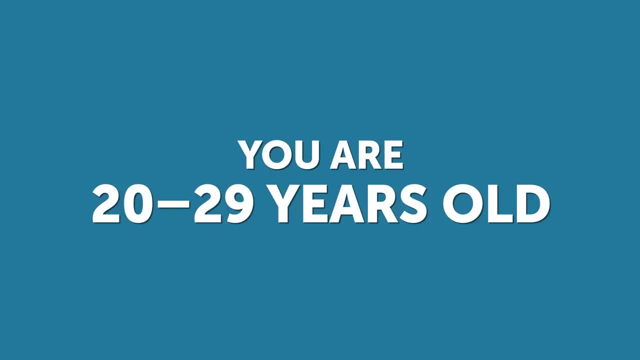 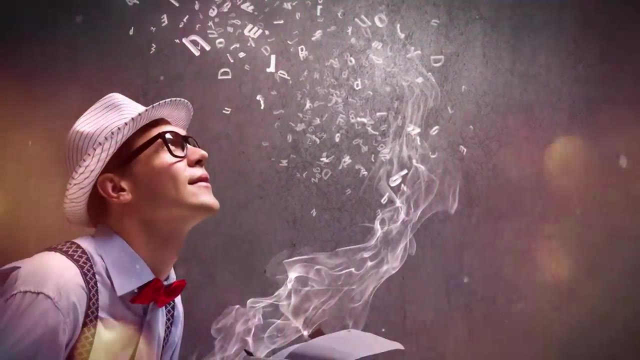 feeling of enthusiasm and love for life through all these years. Keep shining. If your result is 13 to 20 points, you are 20 to 29 years old. You are active, creative and full of life, but you can already call yourself an adult: Childhood and teenage. 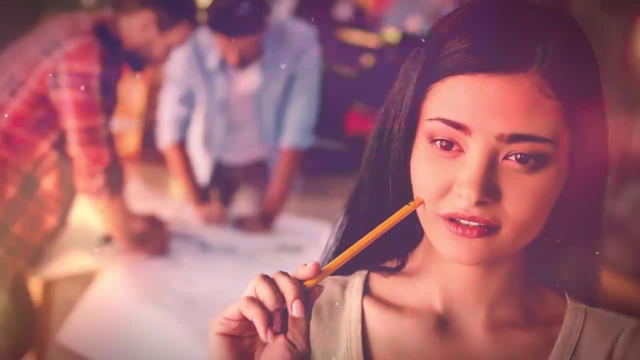 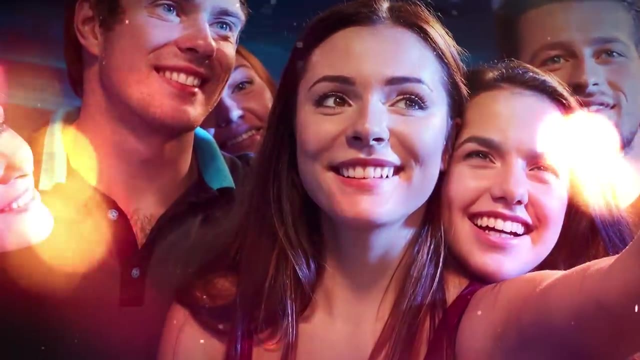 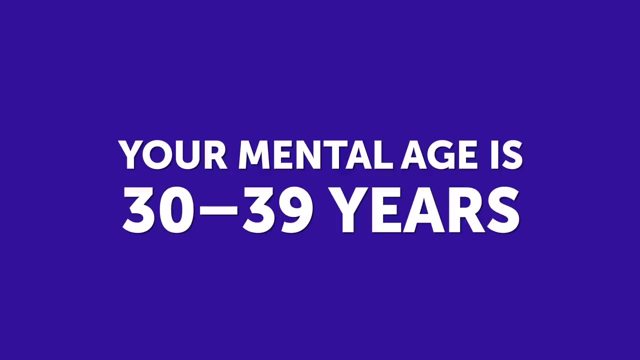 years are over, but you took the best from them and left all the unnecessary stuff behind. It doesn't mean that you're not having fun, though. Your life is just as exciting as it was If all of your points added up to 21 to 28 points. your mental age is 30 to 39 years. 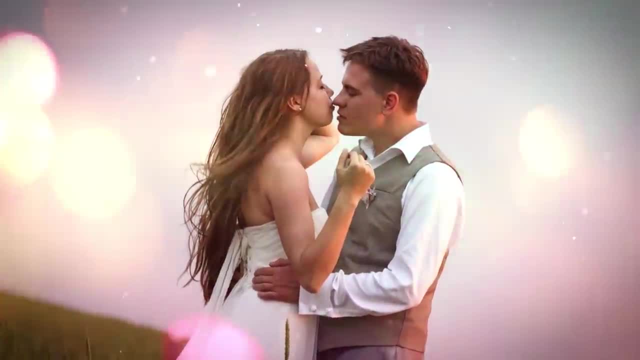 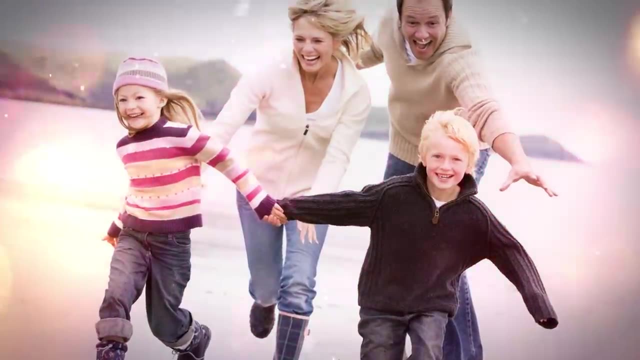 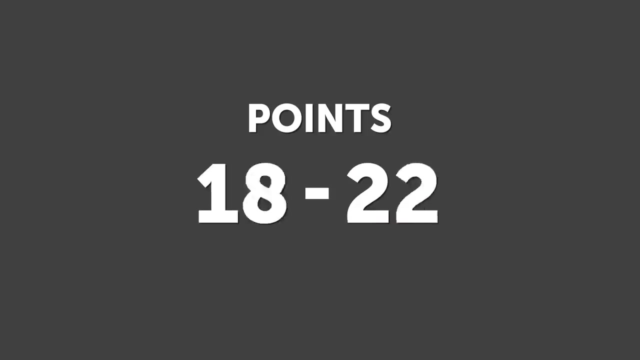 You're still active and curious about new things and ideas, but you're already responsible and thoughtful If you think about it. that's the perfect balance between the children's joy for life and adult independence. The golden mean at its best If your total number of points is 29 to. 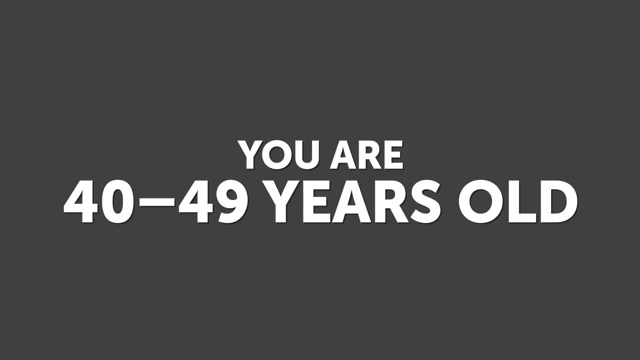 35,, you are 40 to 49 years old. If your total number of points added up to 21 to 28 points, you are 30 to 40 years old. You're mature and experienced and you know exactly how to live. 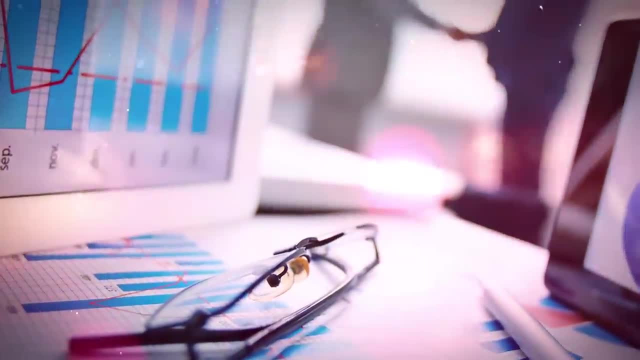 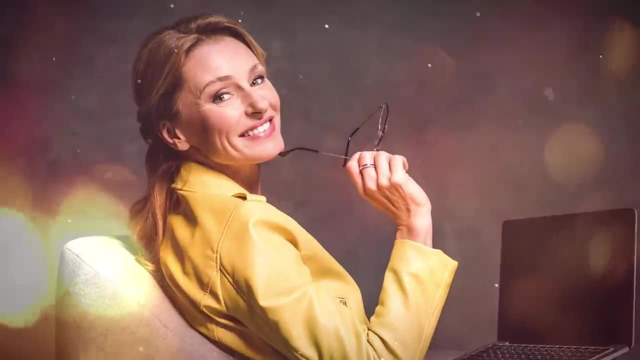 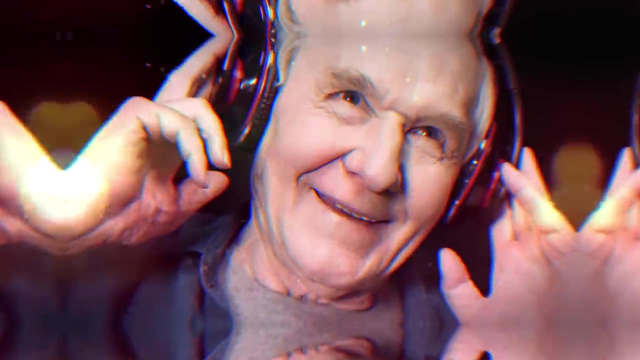 your life. You have no time for nonsense. You're determined and hardworking. You know what you want and how to get it. Continue to be a true inspiration for everyone. around 36 to 40 points means that your mental age is over 50 years, and that's not a bad thing at all. 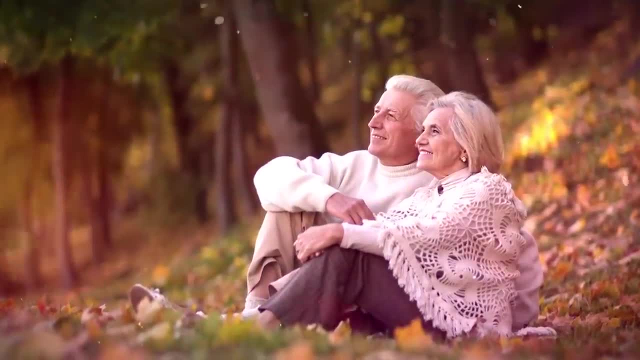 On the contrary, you are wise and calm, You get what life is all about and you hire people to help you. If you have a goal, you have a goal. If you have a goal, you have a goal. What world would you ever want to go to? You can even entrust yourself toWhy. should you do all of this? You should choose not to go to the most point in your life. You're strong, so you will have an advantage. perhaps you'llστε happy, but at the same time you will lose your sense of humor and sort of stiff. You will cheat and lose your.